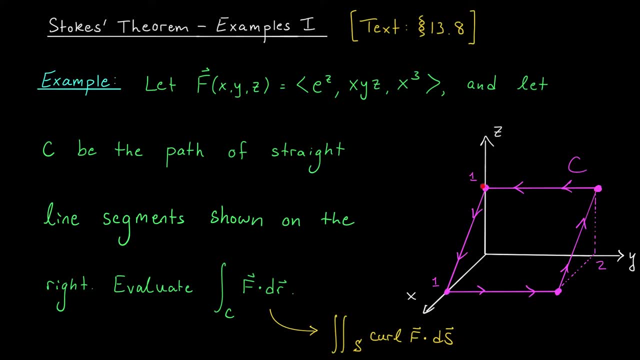 we have to integrate over a surface S whose boundary is this curve C. Now, there are lots of surfaces with this property, but let's keep it simple. We could just take S to be this plane right here. So this is going to be our surface S and our strategy is to compute this. 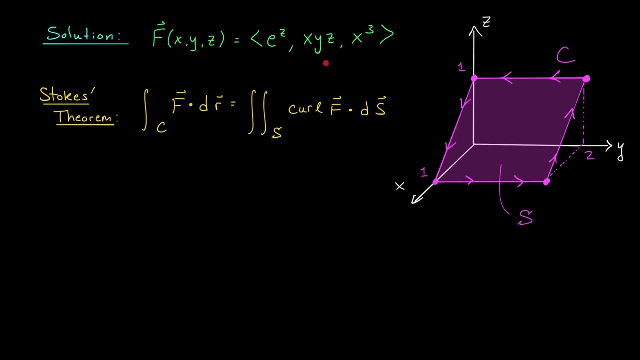 surface integral. Okay, we have our vector, field f, and we're going to apply Stokes' theorem to convert this line integral into a surface integral. If we're going to be computing a surface integral, we should probably know the function that we're going to be integrating. So let's start by 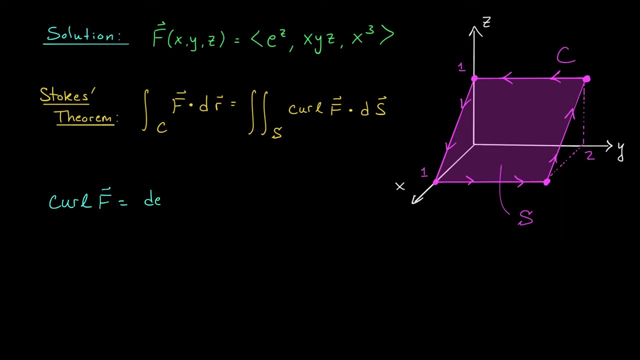 computing the curl of f. So we're going to start by computing the curl of f. So we're going to curl of f. The curl of f is given by the determinant of i, j, k. In the second row we have: 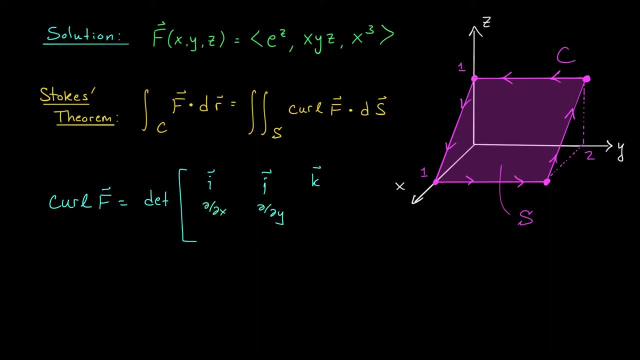 partial by partial x, partial by partial y, partial by partial z. and then finally, our component functions e to the z, x, y, z and x cubed Okay. well, if I look in the i component it looks like. 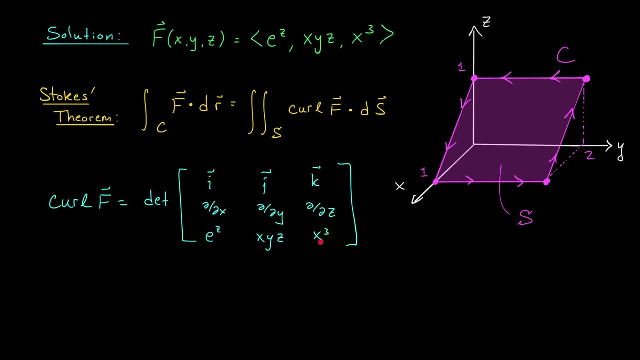 I'm going to be doing partial by partial y of x cubed minus, partial by partial z of x y, z minus x y. We then subtract j times partial by partial x of x cubed minus, partial by partial z of e to the z, and that gives us e to the z minus 3x squared. And then finally we add k times partial. 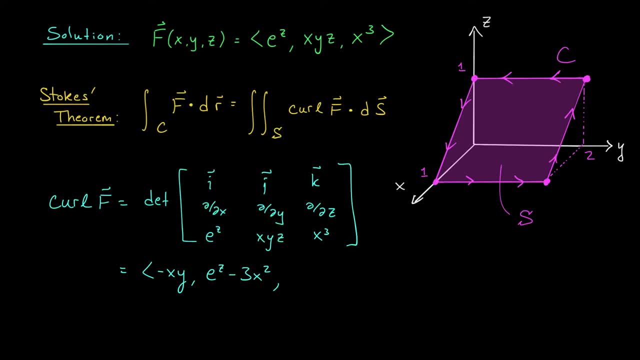 by partial x of x, y z, minus partial by partial y of e to the z, So that's simply y z. All right, the vector field that we're going to be integrating, but we still don't know much about this surface S. If we want to compute this surface integral, we're going to have to find a parametric. 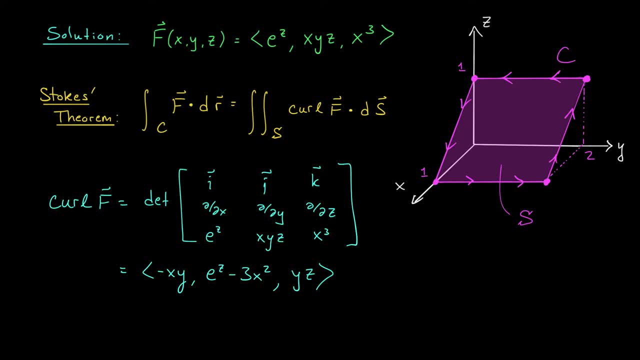 equation that traces our surface. Well, notice that S is part of the plane that passes through these four points. So I guess we could find the equation of the plane by using the techniques. from the very beginning of our course We could say, all right, the plane contains this line. 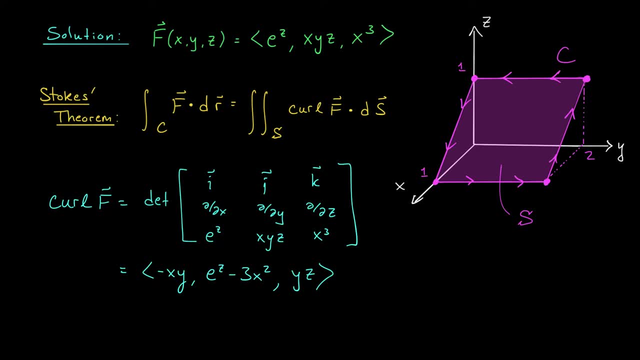 segment and this line segment, and therefore their cross product, is going to give us something that's orthogonal to the plane. But that's a lot of work and I don't think it's necessary here Notice that in our case the plane is really just this line: z equals 1 minus x in the x- z plane. 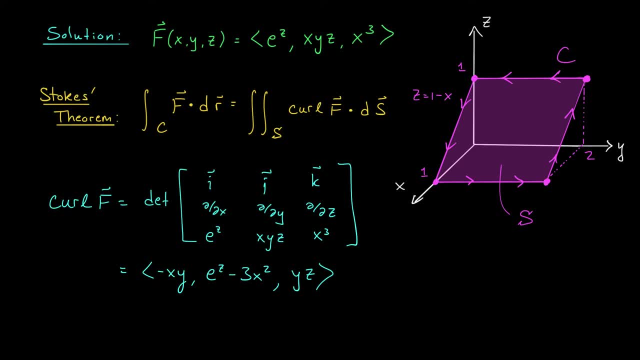 translated parallel to the y-axis. So the equation of the whole plane is: z equals 1 minus x. Of course, S is only part of the plane. It's the part where x is between 0 and 1, and y is between 0 and 2.. 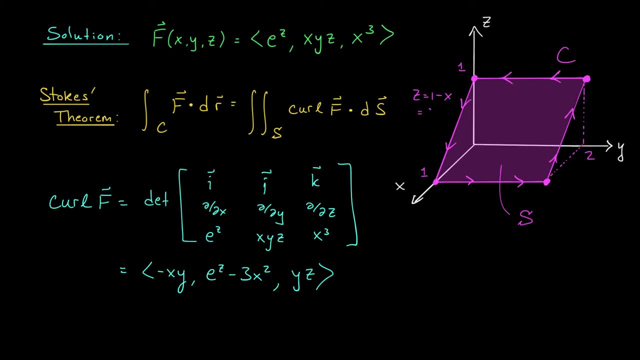 Okay, since S comes from the graph of the function, z equals f of x, y equals 1 minus x, we can use our nice, easy parametrization: S is given by r of x- y equals x, y 1 minus x, where x goes between 0 and 1 and y between 0 and 2.. Now that we have a parametrization, 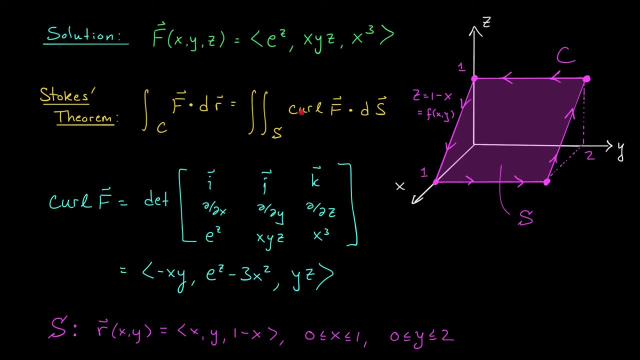 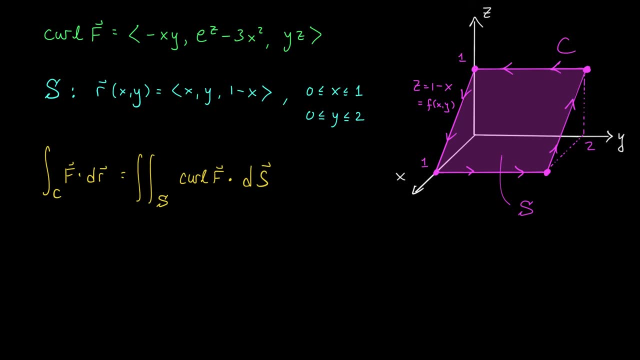 for our surface and the curl of our vector field. we're ready to compute this surface integral. To compute this surface integral, let's think back to our formula. The surface integral of the curl of f throughout S is really the double integral over d, d. here is the set where our parameters 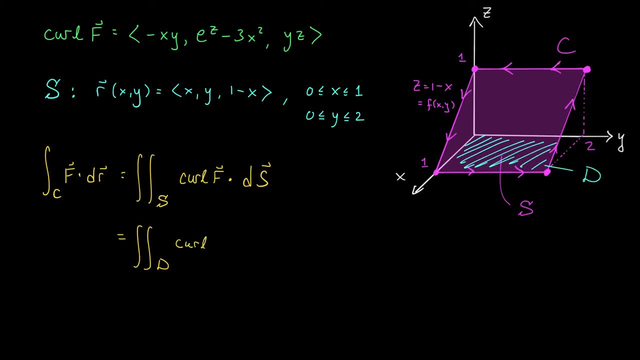 live this set here of curl of f dot r x cross r y, d a Ah. but since we're dealing with the graph of a function here- z equals f of x y- we can compute r x cross r y as minus partial. 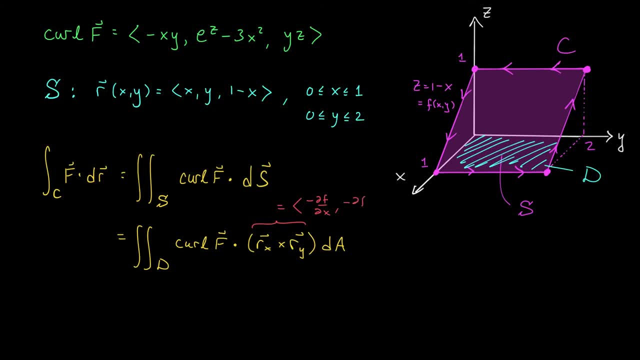 f by partial x minus partial f by partial y and 1.. Now the partial derivative with respect to x here is minus one and the partial derivative with respect to y is zero. so we get the vector one zero one. Now, before moving forward, we should make sure that this normal vector is consistent with: 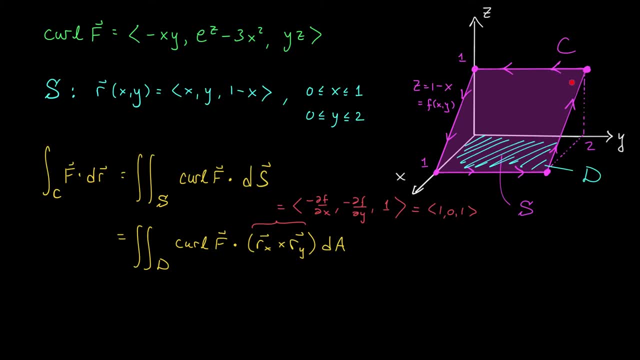 the orientation given to us by C. C is oriented counterclockwise right and if you imagine turning bottle counterclockwise while you're removing the lid, right, The lid is going to come up or away from the bottle. So we're looking for upward orientation. Is that what we have? Yes, it is. 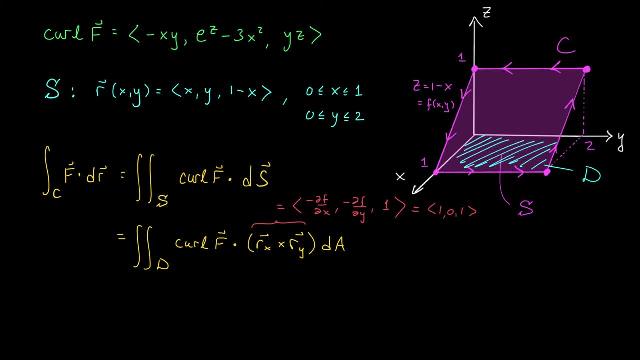 You can see that we have a positive z-coordinate, so this is the correct cross product. Okay, using my bounds on x and y, I can rewrite this integral as the integral from 0 to 1, of the integral from 0 to 2.. And now I'm supposed to take the dot product of the curl of f with this vector 1, 0,.